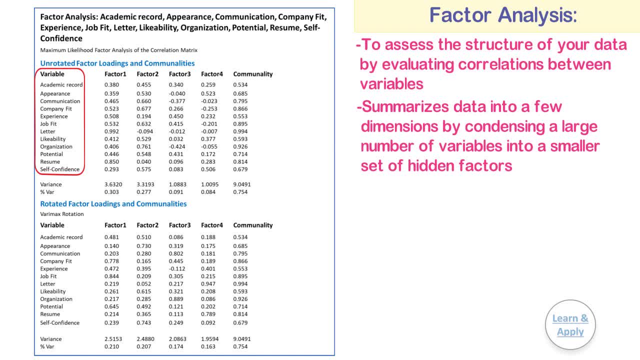 variables into a smaller set of hidden factors that you do not directly measure or observe, but which may be easier to interpret. Using this analysis, you can model each original variable as a linear sequence. Factor analysis is a linear function of these basic factors. Factor analysis is commonly 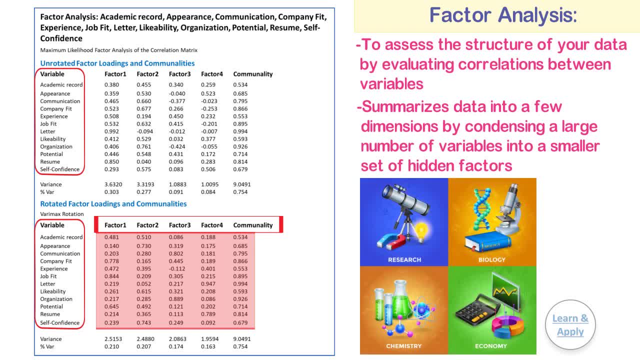 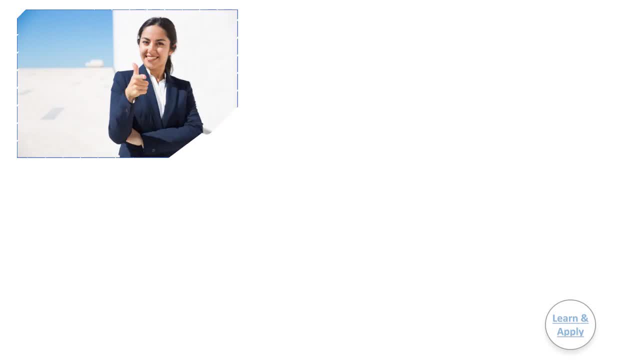 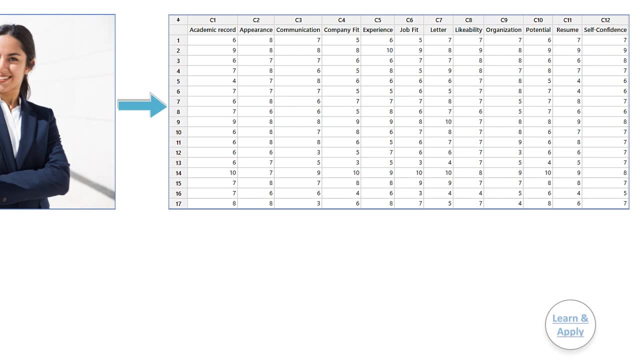 used in the social sciences, market research and other industries that use large datasets. For example, a human resource manager wants to identify the underlying factors that explain the 12 variables that the human resource department measures for each applicant. Human resource employees rate each of the job applicants on various categories. The 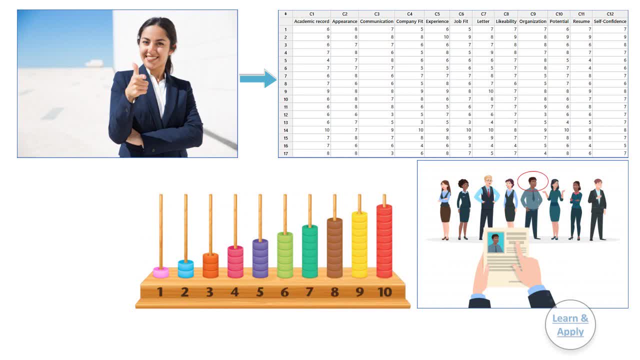 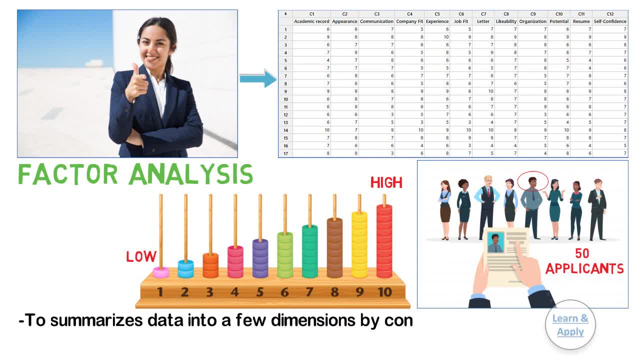 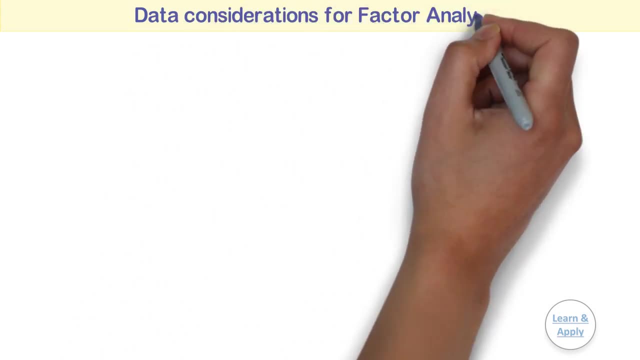 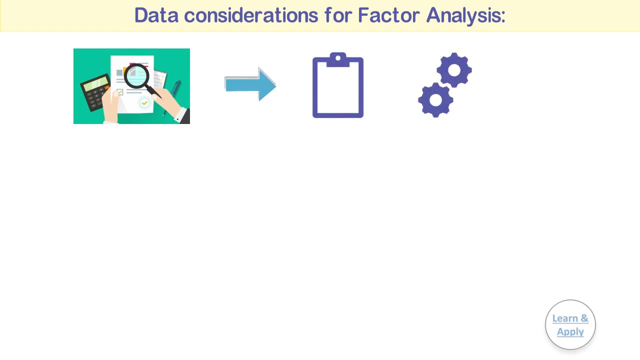 A human resource manager. 그래서 the gross domestic product, gross domestic India and Irene scale is often used in determining 뭐야 meaning of the sex Data considerations for factor analysis. To ensure that your results are valid, consider the following guidelines when you collect the data, perform the analysis and interpret. 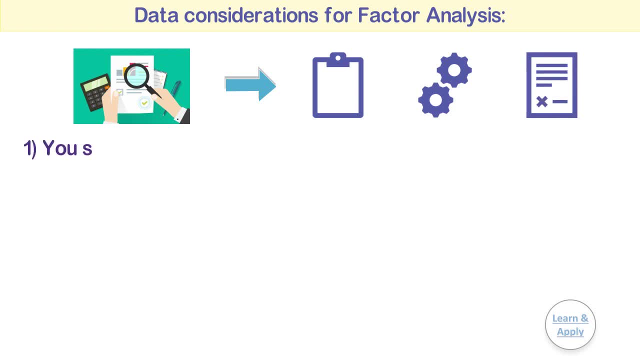 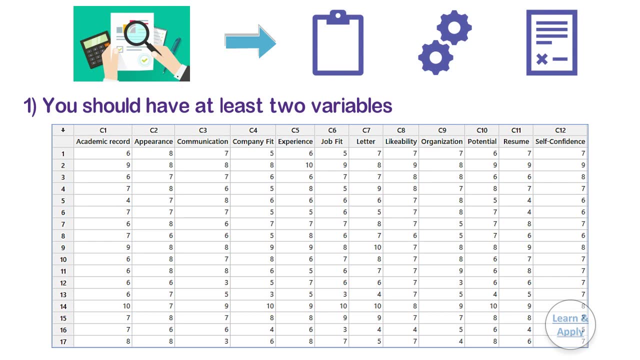 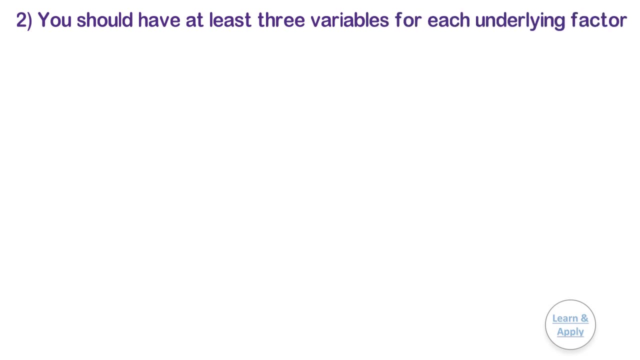 your results. 1. You should have at least two variables and the measurements for each variable should be recorded in separate numeric columns. 2. You should have at least three variables for each underlying factor. Generally, you should not have more than one factor for every three variables in your data. For example: 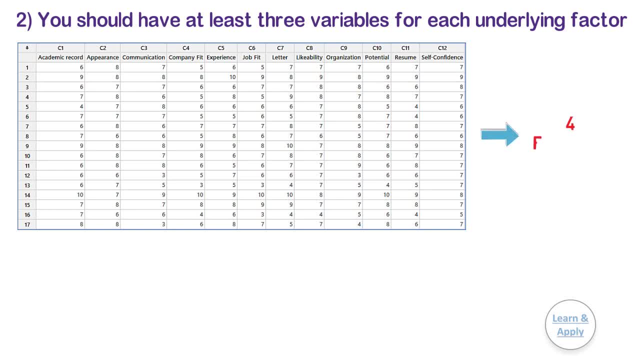 if you are having twelve variables, then you should extract at most four factors. 3. Groups of variables should be highly correlated. For the analysis results to be useful, groups of variables should be highly correlated, with small correlations among variables from different groups. 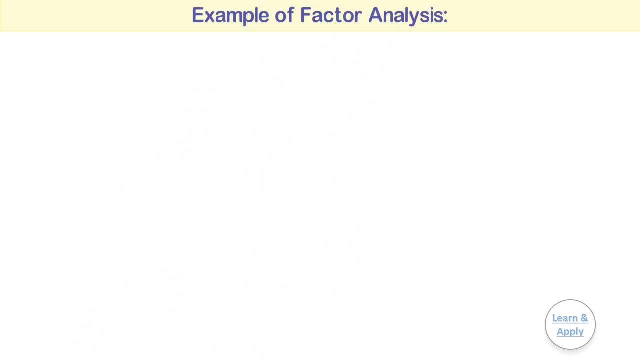 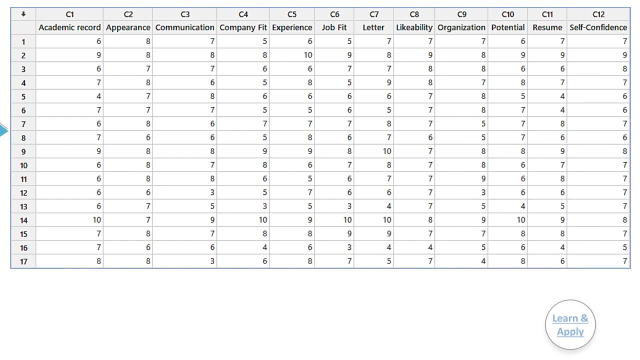 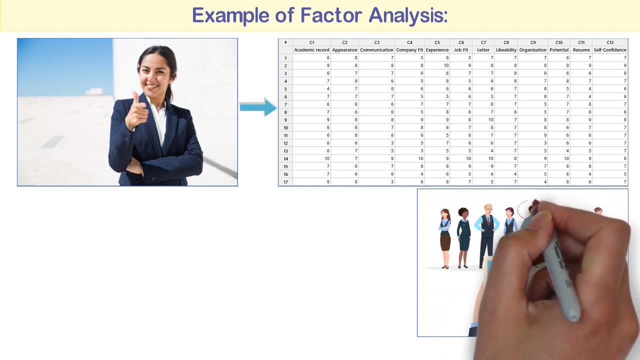 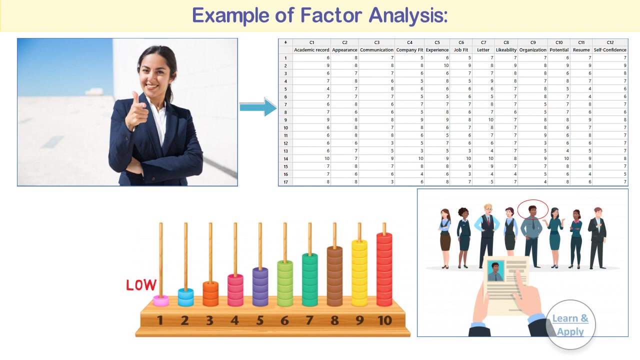 Example of Factor Analysis. Let's continue with the same example. A human resource manager wants to identify the underlying factors that explain the twelve variables that the human resource department measures for each applicant. Human resource employees rate each of the job applicants on various characteristics, using a scale of 1 as a low, through 10 as 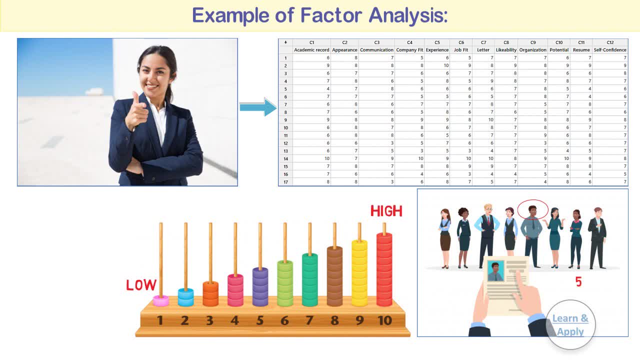 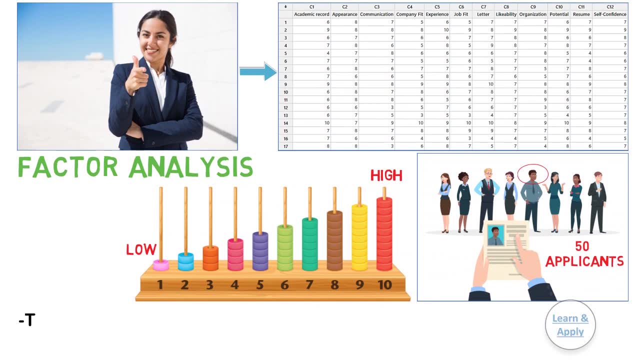 a high. The manager collects the ratings for 50 job applicants. Here the human resource manager performs a factor analysis to summarize this data into a few dimensions by considering a large number of variables into a smaller set of hidden factors that you do not directly measure or observe, but which may be easier to interpret. 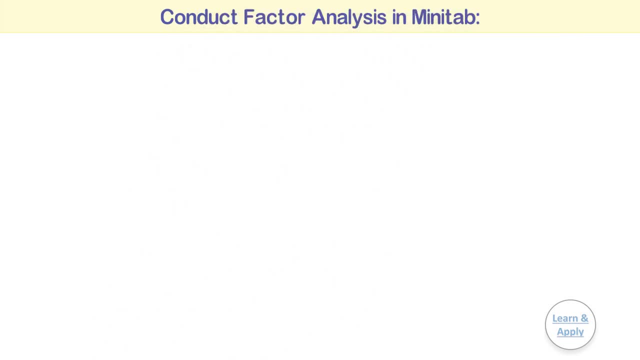 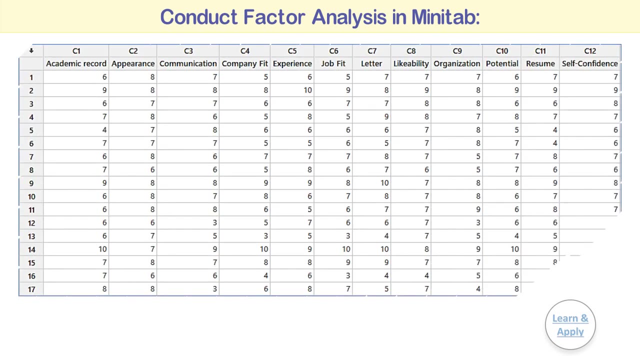 Conduct a Factor Analysis in Minitab. To conduct a factor analysis in Minitab, please follow these steps: 1. Enter or copy the data to the Minitab worksheet, With the data for 1 variable in one column, as shown in the picture. 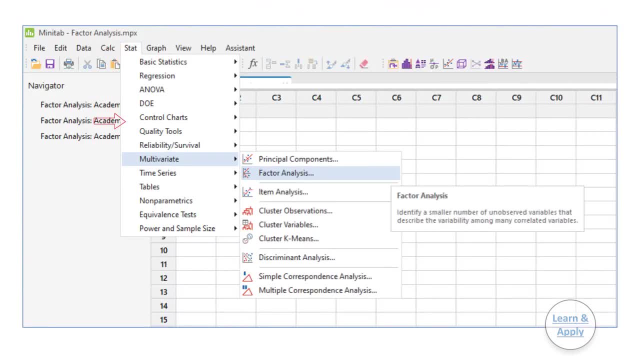 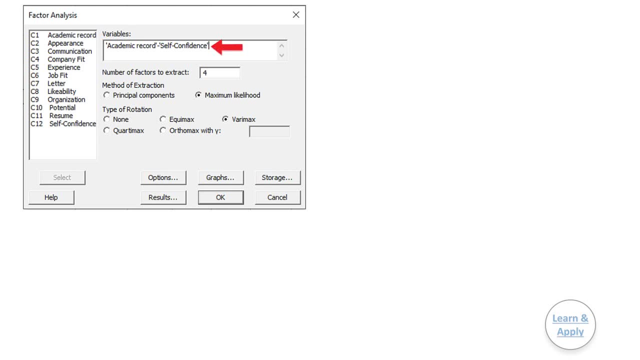 2. Select clair multivariate and then factor analysis. 3. In variables: enter c1 to c12. 4. In Number of Factors to Extract: enter. 4. Here enter the number of factors to extract from the data. The number of factors to extract must be at least c12, and can be found in the following options. For example, spread a turn유. Canadian rule reads that a number of factors must be one in each column. If the factors are non geeky then this number can be omitted. It is a valid, we nói. 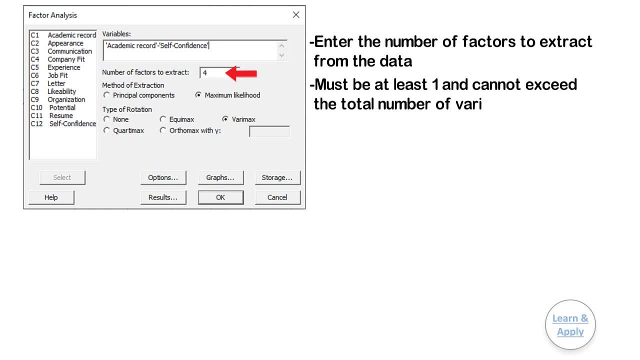 one and cannot exceed the total number of variables. For best results, you should not have more than one factor for every three variables in your data. In our example, as we are having 12 variables, we should extract at most 4 factors If you. 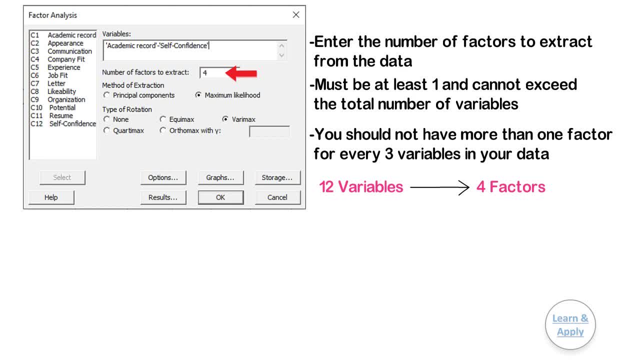 do not know how many number of factors to extract, then leave the field as blank. 5. Under Method of extraction: select Maximum likelihood. Select the correct method to extract the factors. Principal components: Select this option if you do not know the number of factors to extract. 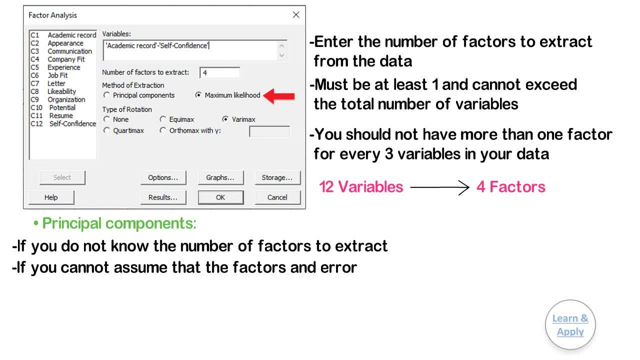 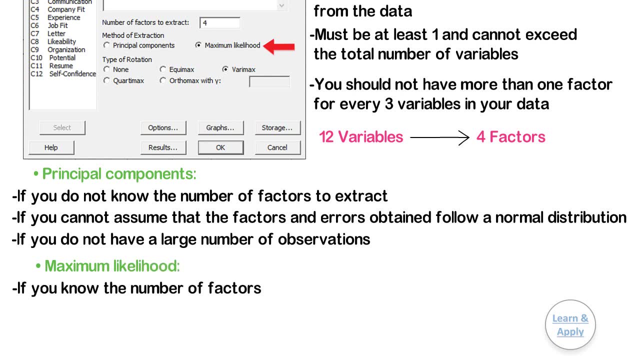 or if you cannot assume that the factors and errors obtained after fitting the factor model follows a normal distribution or you do not have a large number of observations Maximum likelihood. Select this option if you know the number of factors to extract or you can assume that. 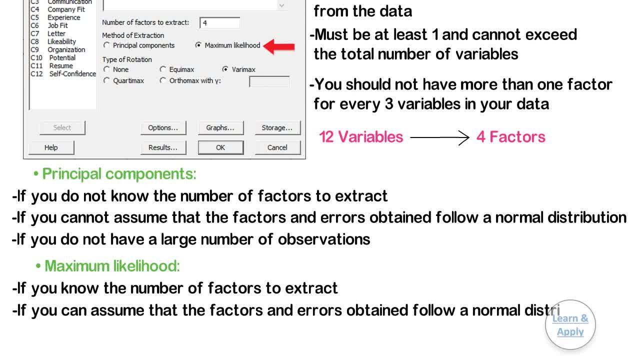 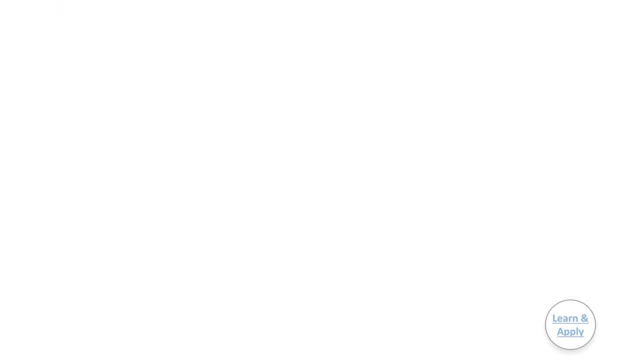 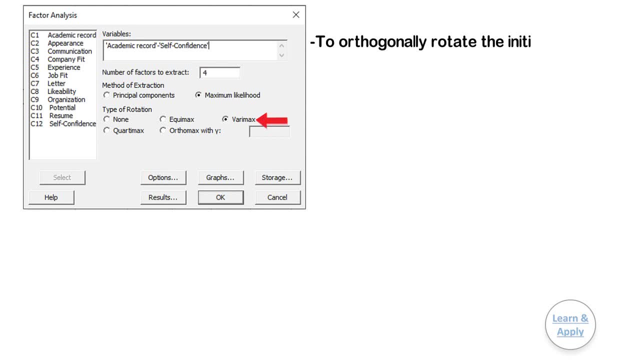 the factors and errors obtained after fitting. the factor model follows a normal distribution and you have a reasonably large data set. 6. Under Type of rotation: select Varymax. Select an option to orthogonally rotate the initial factor. loadings Minitab rotates the axis to give you a different perspective. 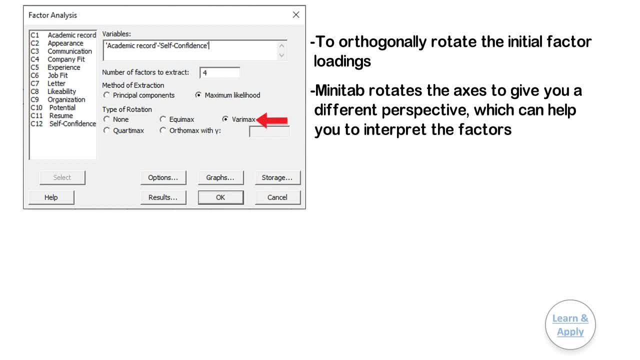 This can help you to interpret the factors. The original factor loadings are often difficult to interpret. The rotation usually creates a simple factor structure and makes the factors more clearly distinguishable. Rotation also tends to remove general factors that load highly on all the variables. 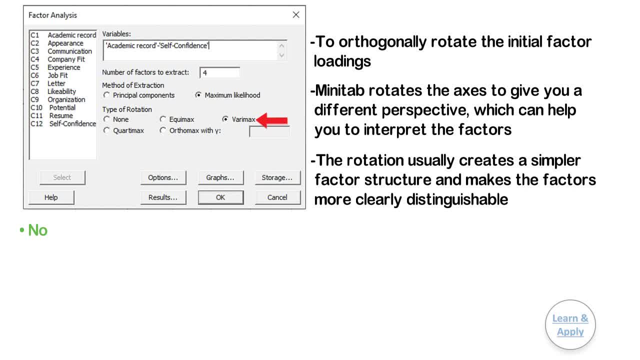 There are below options to select the type of rotation: None, do not rotate the loading. 7. Under Type of rotation: select Varymax. Select the type of rotation: None, do not rotate the loading. 8. Under Type of rotation: select Varymax. Select the type of rotation. None, do not rotate. 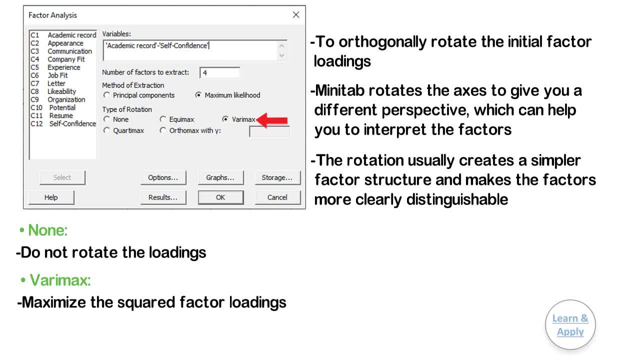 the loading. 9. Under Type of rotation: select Varymax. Select the type of rotation. None, do not rotate the loading. 10. Under Type of rotation: select Varymax. Select the type of rotation. None, do not rotate. 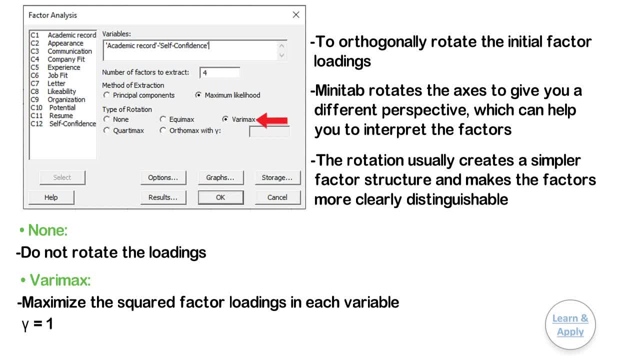 the loading. 11. Under Type of rotation: select Varymax. Select the type of rotation. None, do not rotate the loading. 12. Under Type of rotation: select Varymax. Select the type of rotation. None, do not rotate. 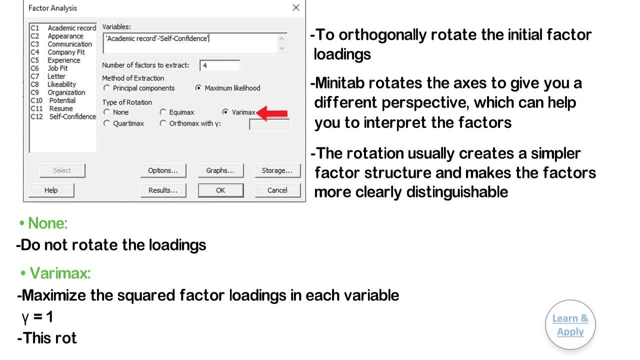 the loading. 13. Under Type of rotation: select Varymax. Select the type of rotation. None, do not rotate the loading. 14. Under Type of rotation: select Varymax. Select the type of rotation. None, do not rotate. 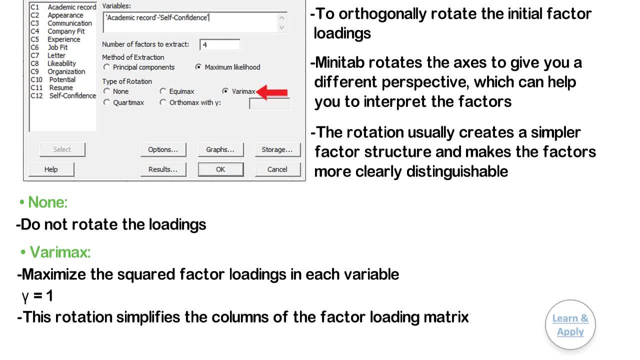 the loading. 15.. Under Type of rotation: select Varymax. Select the type of rotation. None, do not rotate the loading. 16. Under Type of rotation: select Varymax. Select the type of rotation. None, do not rotate. 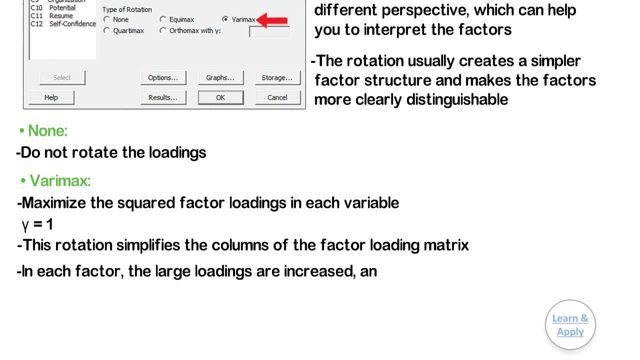 the loading. 17.. Under Type of rotation: select Varymax. Select the type of rotation. None, do not rotate the loading. 18.. Under Type of rotation: select Varymax. Select the type of rotation. None, do not rotate. 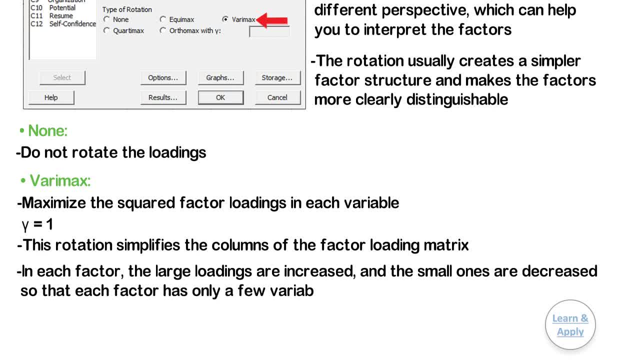 the loading. 19.. Under Type of rotation: select Varymax. Select the type of rotation. None, do not rotate the loading. 20. Under Type of rotation: select Varymax. Select the type of rotation. None, do not rotate. 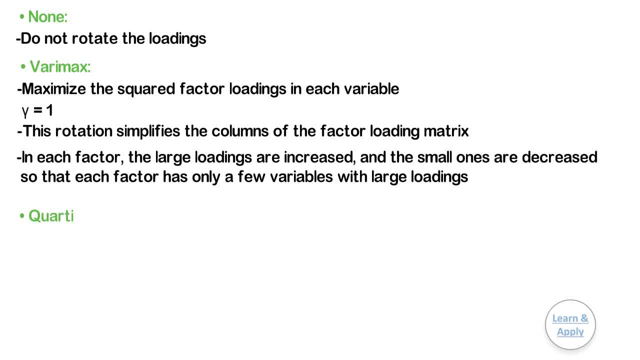 the loading. 21. Under Type of rotation: select Varymax. Select the type of rotation. None, do not rotate the loading. 22. Under Type of rotation: select Varymax. Select the type of rotation. None, do not rotate. 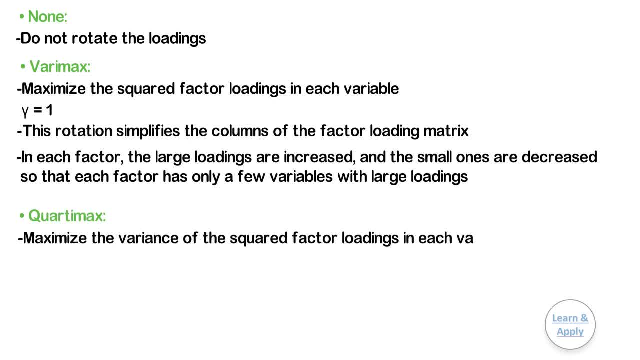 the loading. 23. Under Type of rotation: select Varymax. Select the type of rotation. None, do not rotate the loading. 24. Under Type of rotation: select Varymax. Select the type of rotation. None, do not rotate. 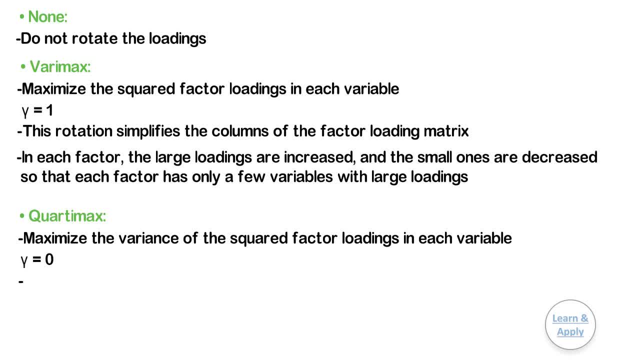 the loading 25.. Under Type of rotation: select Varymax. Select the type of rotation. None, do not rotate the loading. 26.. Under Type of rotation: select Varymax. Select the type of rotation. None, do not rotate. 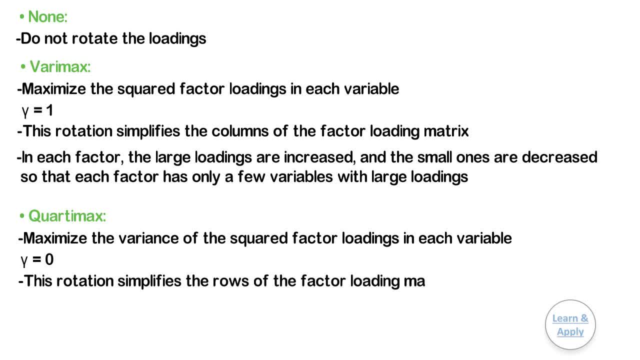 the loading 27.. Under Type of rotation: select Varymax. Select the type of rotation. None, do not rotate the loading. 28.. Under Type of rotation: select Varymax. Select the type of rotation. None, do not rotate. 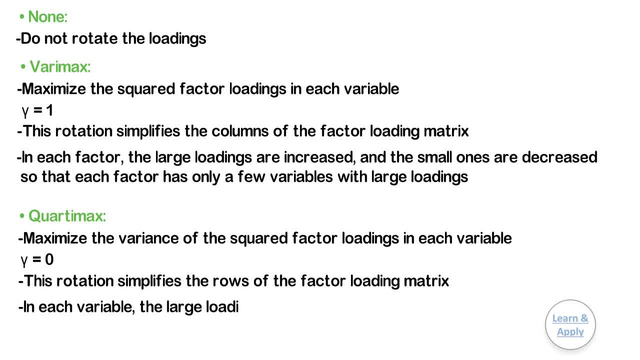 the loading 29.. Under Type of rotation: select: Varymax. Select the type of rotation: None. do not rotate the loading 30.. Under Type of rotation: select Varymax. Select the type of rotation. None, do not rotate. 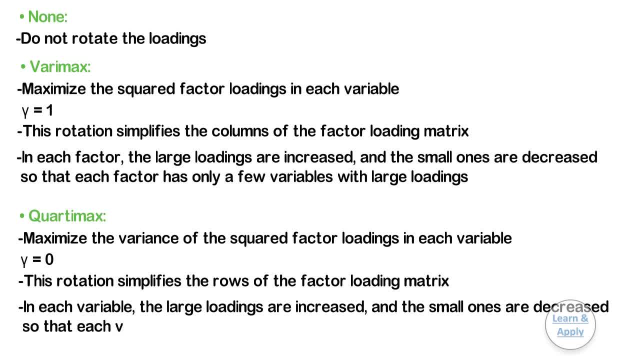 the loading. 31.. Under Type of rotation: select Varymax. Select the type of rotation. None, do not rotate the loading. 32.. Under Type of rotation: select Varymax. Select the type of rotation. None, do not rotate. 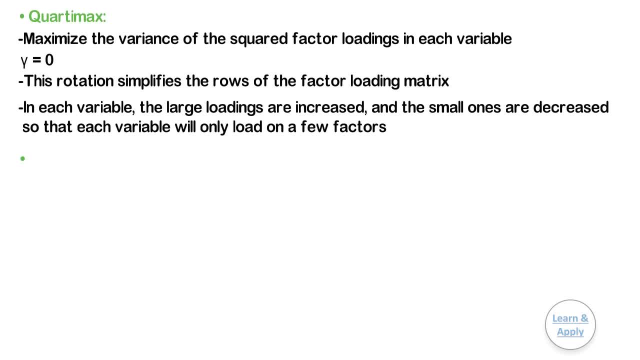 the loading 33.. Under Type of rotation: select Varymax. Select the type of rotation. None, do not rotate the loading. 34.. Under Type of rotation: select Varymax. Select the type of rotation. None, do not rotate. 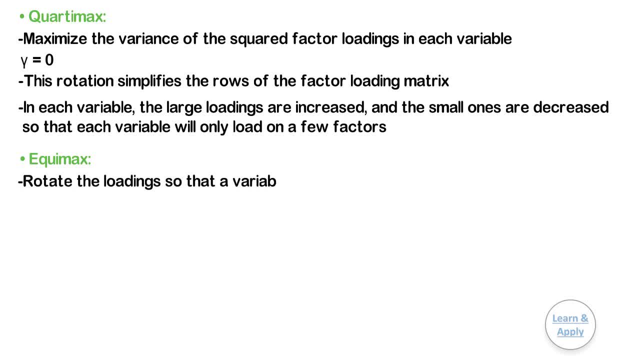 the loading 35.. Under Type of rotation: select Varymax. Select the type of rotation: None. do not rotate the loading 36.. Under Type of rotation: select Varymax. Select the type of rotation: None. do not rotate. 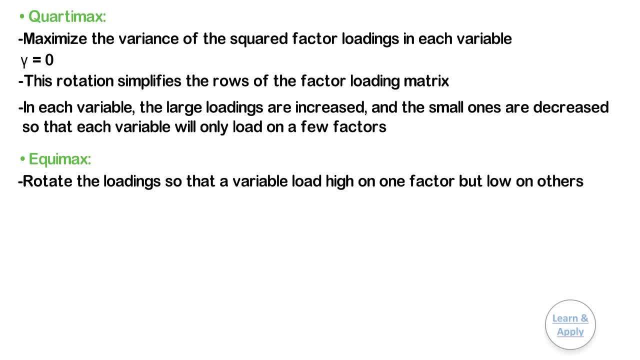 the loading 37.. Under Type of rotation: select Varymax. Select the type of rotation: None. do not rotate the loading 38.. Under Type of rotation: select Varymax. Select the type of rotation. None, do not rotate. 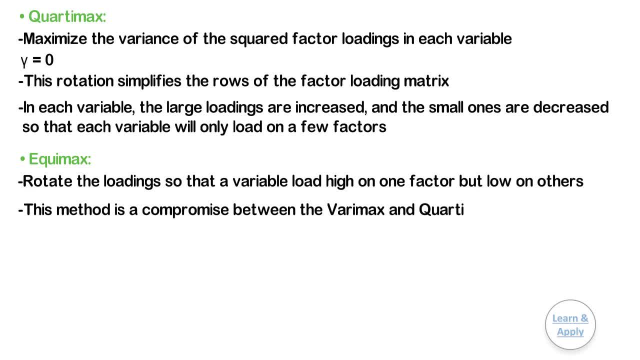 the loading 39.. Under Type of rotation: select Varymax. Select the type of rotation: None. do not rotate the loading 40.. Under Type of rotation: select Varymax. Select the type of rotation. None, do not rotate. 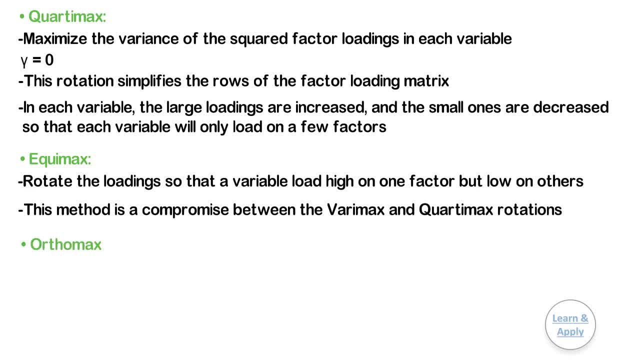 the loading. 41.. Under Type of rotation: select Varymax. Select the type of rotation: None. do not rotate the loading. 42.. Under Type of rotation: select Varymax. Select the type of rotation. None, do not rotate. 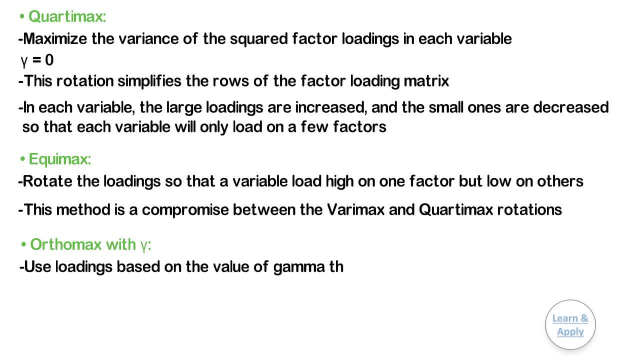 the loading 43.. Under Type of rotation: select Varymax. Select the type of rotation: None. do not rotate the loading. 44.. Under Type of rotation: select Varymax. Select the type of rotation: None, do not rotate. 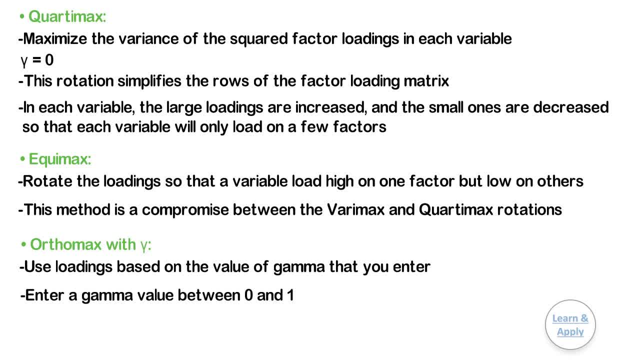 the loading. 45.. Under Type of rotation: select Varymax. Select the type of rotation: None. do not rotate the loading. 46.. Under Type of rotation: select Varymax. Select the type of rotation. None, do not rotate. 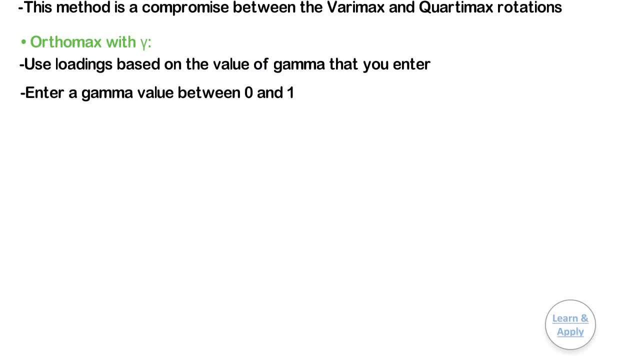 the loading 47.. Under Type of rotation: select Varymax. Select the type of rotation: None, do not rotate the loading 48.. Under Type of rotation: select Varymax. Select the type of rotation. None, do not rotate. 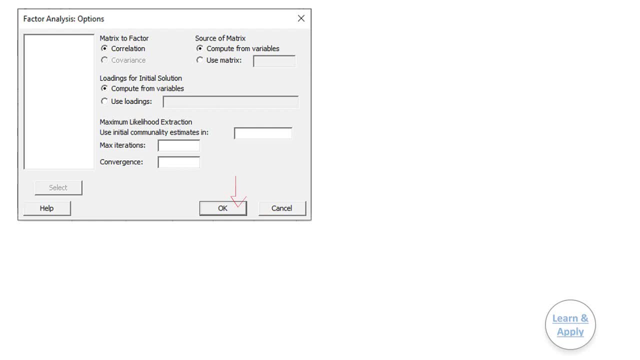 the loading 49.. Under Type of rotation: select Varymax. Select the type of rotation: None. do not rotate the loading 50.. Under Type of rotation: select Varymax. Select the type of rotation. None, do not rotate. 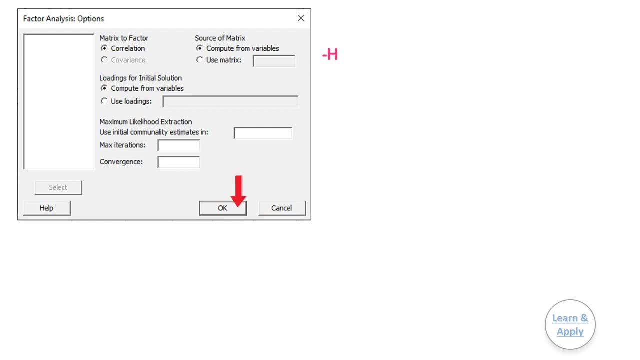 the loading 51.. Under Type of rotation: select Varymax. Select the type of rotation: None. do not rotate the loading. 52.. Under Type of rotation: select Varymax. Select the type of rotation. None, do not rotate. 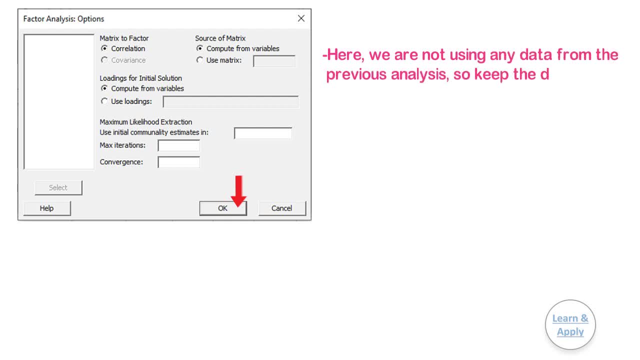 the loading. 53.. Under Type of rotation: select Varymax. Select the type of rotation: None. do not rotate the loading. 54.. Under Type of rotation: select Varymax. Select the type of rotation. None, do not rotate. 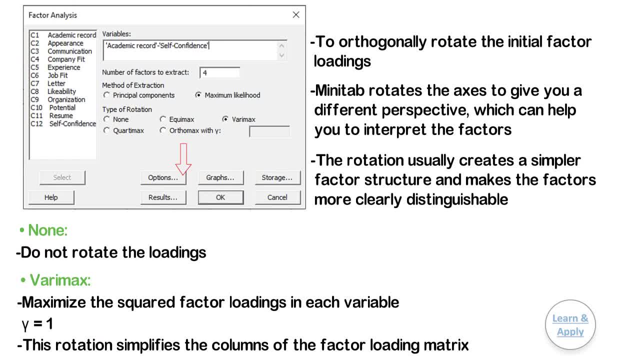 the loading 55.. Under Type of rotation: select Varymax. Select the type of rotation: None. do not rotate the loading 56.. Under Type of rotation: select Varymax. Select the type of rotation: None, do not rotate. 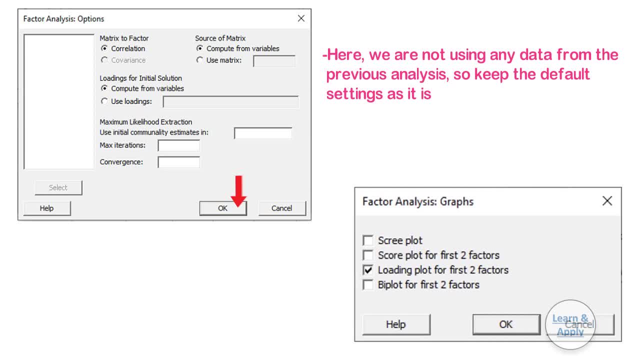 the loading. 57.. Under Type of rotation: select Varymax. Select the type of rotation: None. do not rotate the loading. 58.. Under Type of rotation: select Varymax. Select the type of rotation. None, do not rotate. 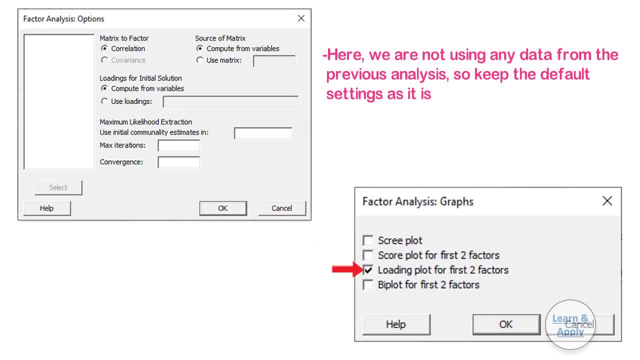 the loading. 59.. Under Type of rotation: select Varymax. Select the type of rotation: None. do not rotate the loading. 60.. Under Type of rotation: select Varymax. Select the type of rotation. None, do not rotate. 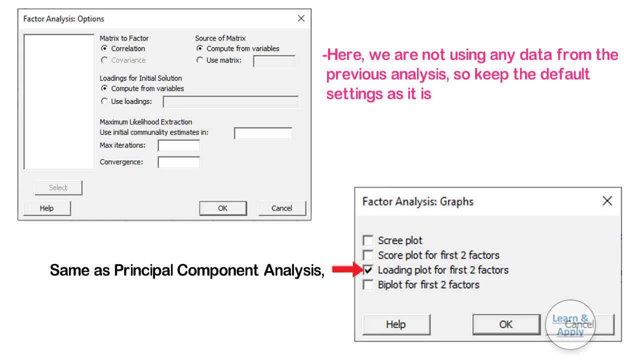 the loading. 61.. Under Type of rotation: select Varymax. Select the type of rotation: None. do not rotate the loading. 62.. Under Type of rotation: select Varymax. Select the type of rotation. None, do not rotate. 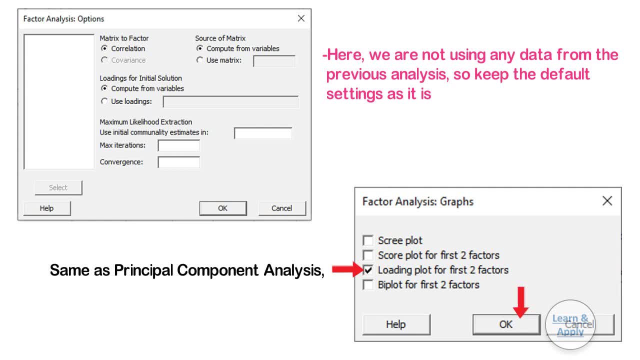 the loading 63.. Under Type of rotation: select Varymax. Select the type of rotation: None. do not rotate the loading 64.. Under Type of rotation: select Varymax. Select the type of rotation: None. do not rotate. 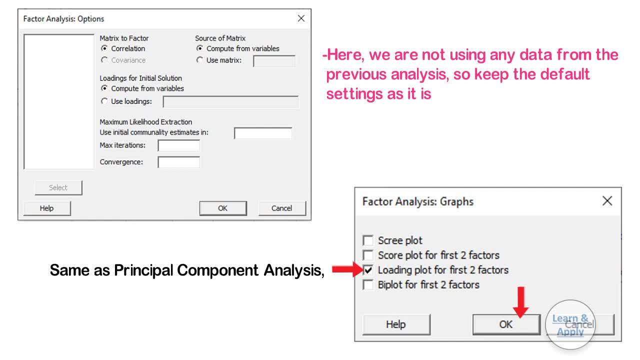 the loading 65.. Under Type of rotation: select Varymax. Select the type of rotation: None. do not rotate the loading 66.. Under Type of rotation: select Varymax. Select the type of rotation. None, do not rotate. the loading 67.. Under Type of rotation: select Varymax. Select the type of rotation: None. do not rotate the loading 68.. Under Type of rotation: select Varymax. Select the type of rotation. None, do not rotate. 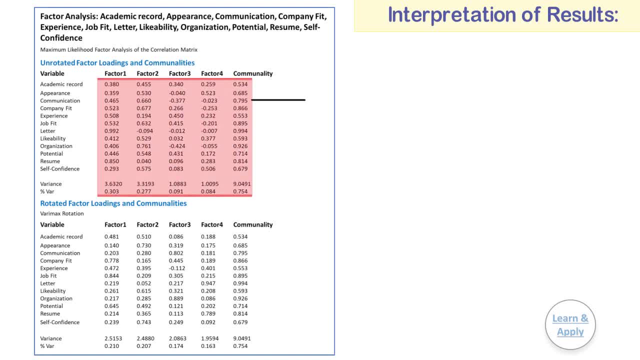 the loading 69.. Under Type of rotation: select Varymax. Select the type of rotation: None. do not rotate the loading. 70.. Under Type of rotation: select Varymax. Select the type of rotation. None, do not rotate. 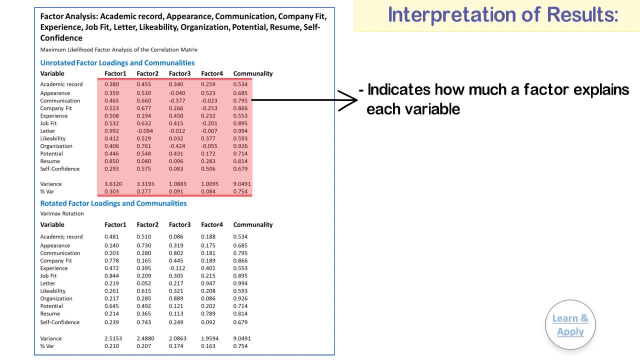 the loading. 71.. Under Type of rotation: select Varymax. Select the type of rotation: None. do not rotate the loading. 72.. Under Type of rotation: select Varymax. Select the type of rotation. None, do not rotate. 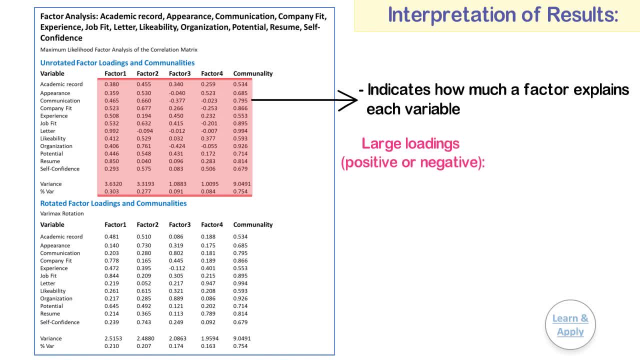 the loading 73.. Under Type of rotation: select Varymax. Select the type of rotation: None. do not rotate the loading. 74.. Under Type of rotation: select Varymax. Select the type of rotation. None. do not rotate. 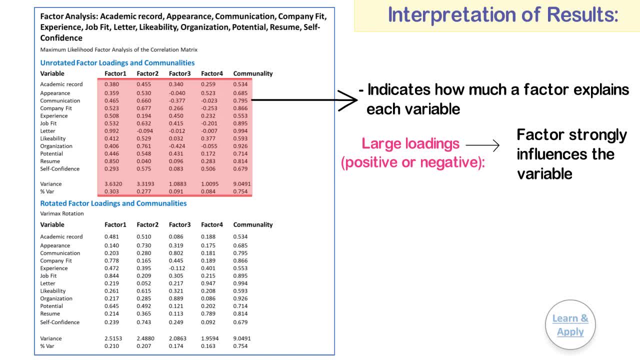 the loading 75.. Under Type of rotation: select Varymax. Select the type of rotation: None. do not rotate the loading 76.. Under Type of rotation: select Varymax. Select the type of rotation. None, do not rotate. 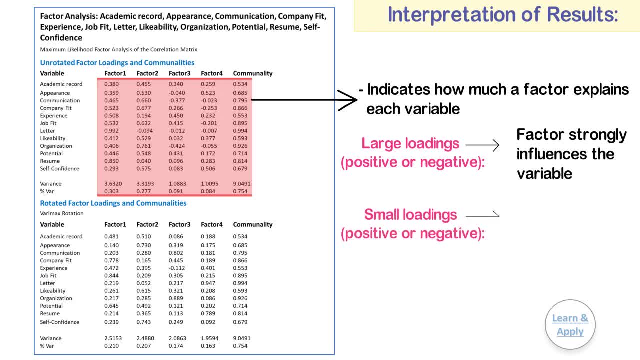 the loading 77.. Under Type of rotation: select Varymax. Select the type of rotation: None. do not rotate the loading. 78.. Under Type of rotation: select Varymax. Select the type of rotation. None, do not rotate. 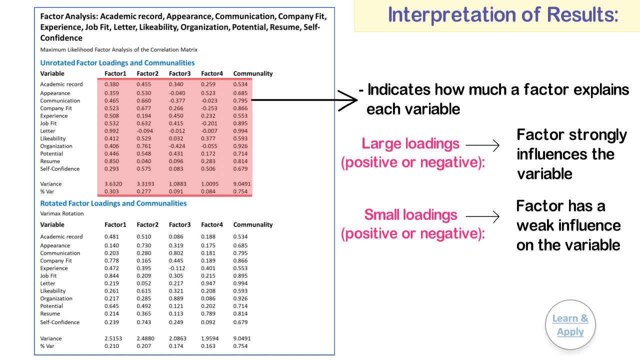 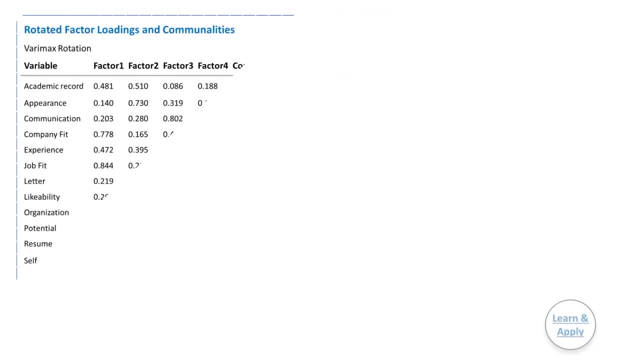 the loading influence on the variable. Unrotated factor loadings are often difficult to interpret. Factor rotation simplifies the loading structure and makes the factor loadings easier to interpret Using the rotated factor loadings. the manager concludes the following Here: company fit, job fit and potential have large positive loadings on factor. 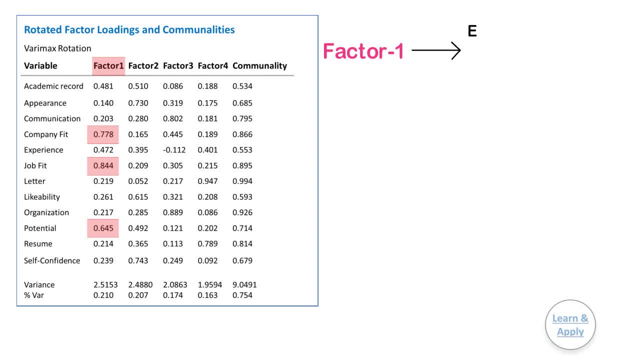 1.. So this factor describes employee fit and potential for growth in the company. Appearance, likability and self-confidence have large positive loadings on factor 2.. So this factor describes personal qualities. Communication and organization have large positive loadings on factor 3.. 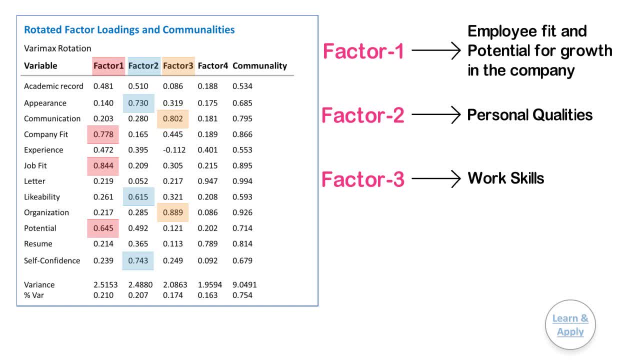 So this factor describes work skills And later and resume have large positive loadings on factor 4.. So this factor describes writing skills. Together, all four factors explain 0.754 or 75.4% of the variation in the data. 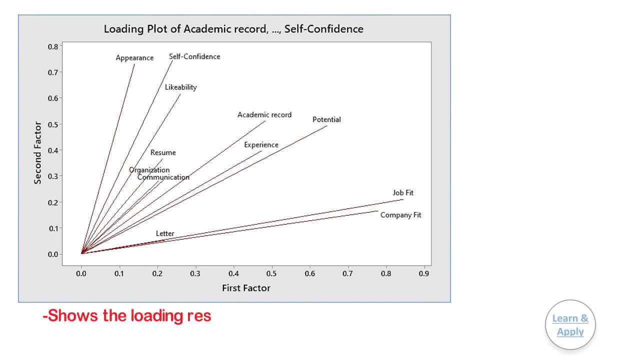 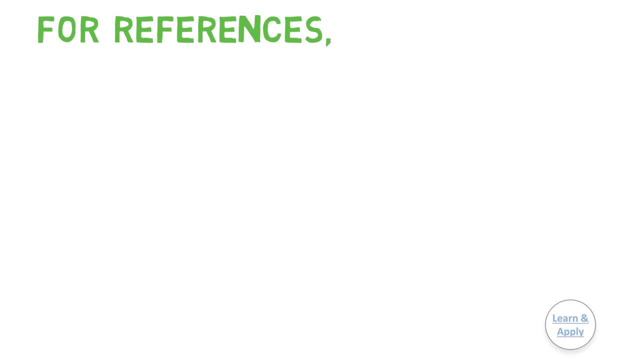 The loading plot visually shows the loading results for the first two factors. This is all about the detailed illustration of factor analysis. We will see the next type of multivariate tools with a practical example in the next video. For references, I have taken some part of this very detailed content from Minitab. 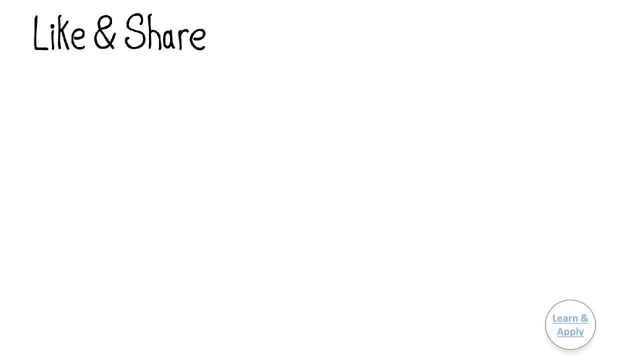 Now to end. please like this video. if you found it useful, add your valuable comments and share this video to your friends and colleagues to improve and refresh their knowledge. If you want to get updates of such videos from my channel, please do not forget to subscribe. 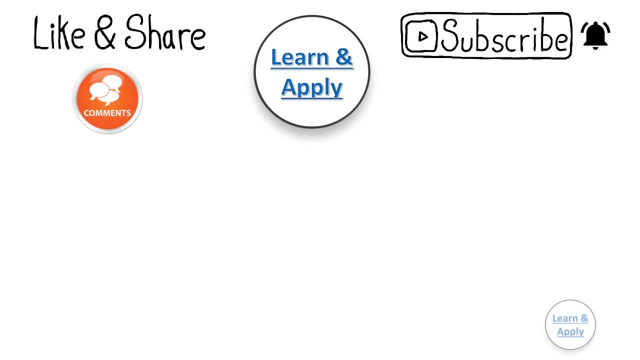 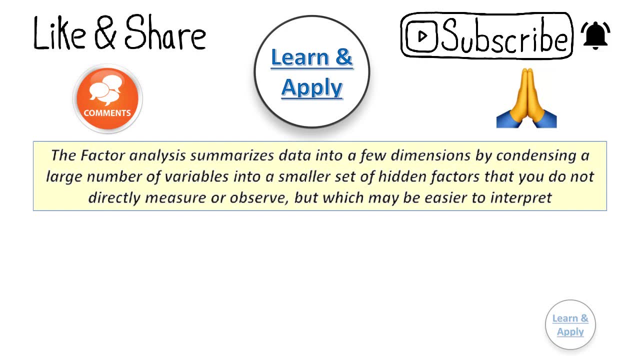 it and click on the bell icon and select to get all notifications. And finally, thank you for watching. See you in the next video. 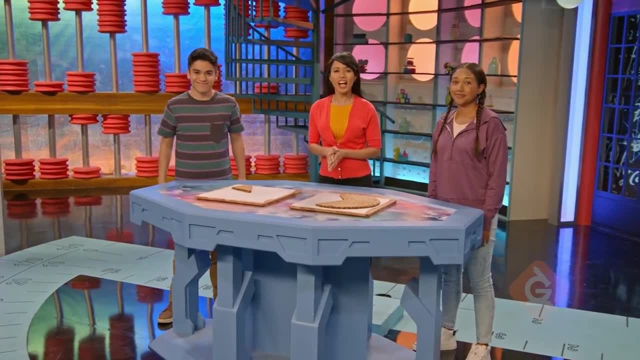 Let's see how adding fractions with unlike denominators can help us eat giant cookies. 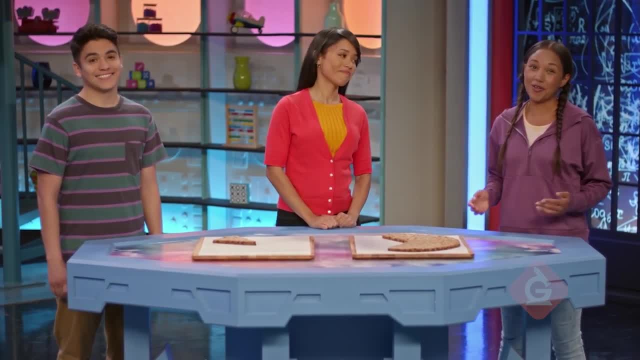 These cookies were so big that we couldn't eat them all. Marcos has 1 9th of a cookie left, 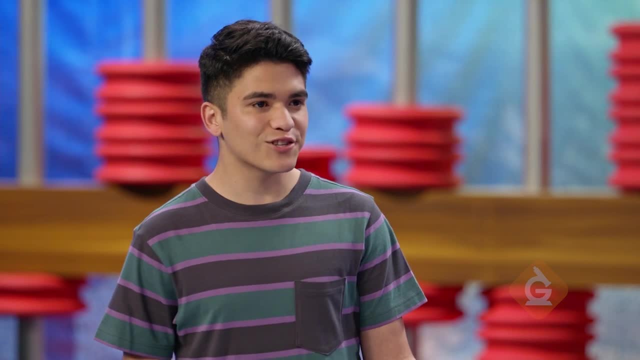 and I have 2 3rds of a cookie left. To find the total, we could add 1 9th plus 2 3rds. 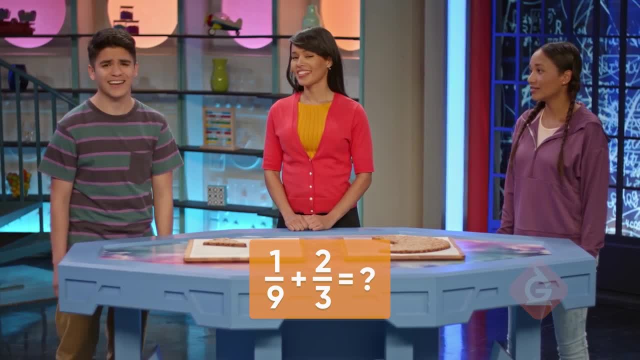 But the denominators aren't the same, so I'm not sure how to add them. One way to add these fractions 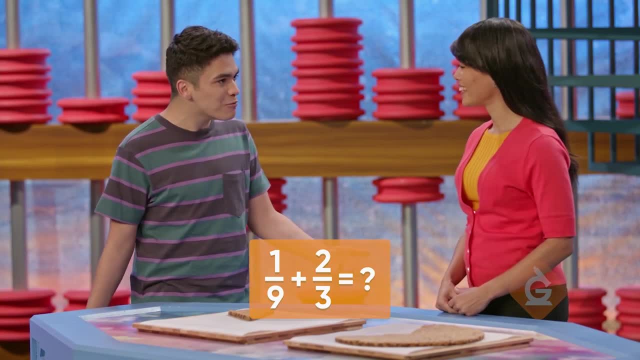 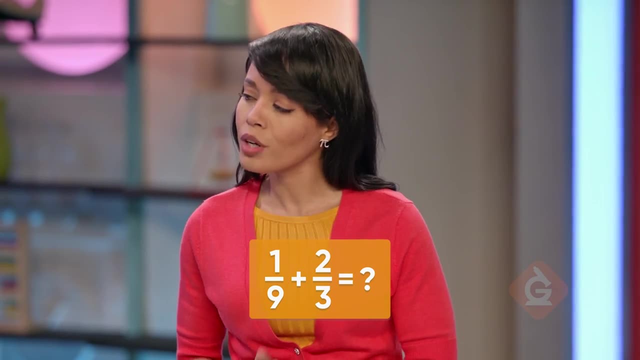 We can find equivalent fractions and see if we can get the same denominators. Exactly. Since 2 3rds has a smaller denominator, why don't you start by finding equivalent fractions for it? 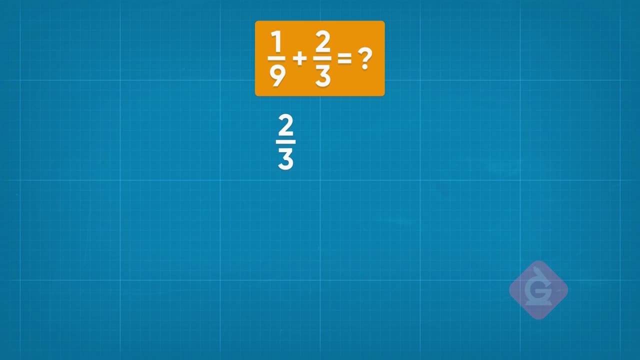 Okay. Well, if we multiply the numerator and denominator by 2, it becomes 4 6ths. And if we multiply the numerator and denominator by 3, we get 6 9ths. That's it. 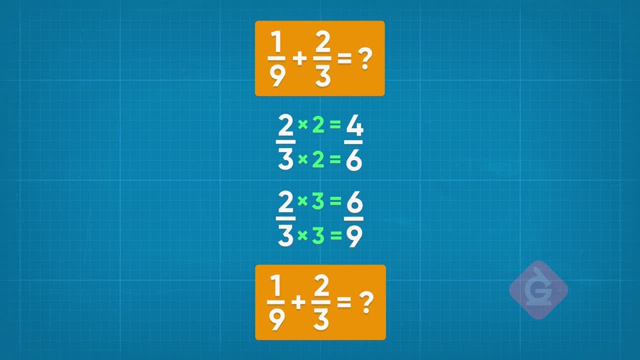 Since 6 9ths is equivalent to 2 3rds, we can use 6 9ths in the problem.